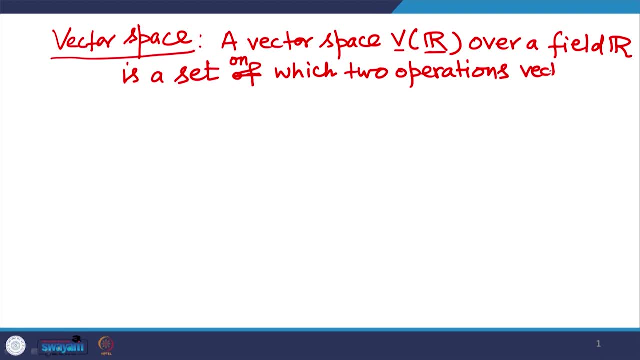 us say vector addition, denoted by plus. So this plus is defining the vector addition, and scalar multiplication, let us denote it by dot, are defined. So these two operations are well defined. on V and R, such that The first property, the set of vector V, together with the operation addition of vectors, forms: 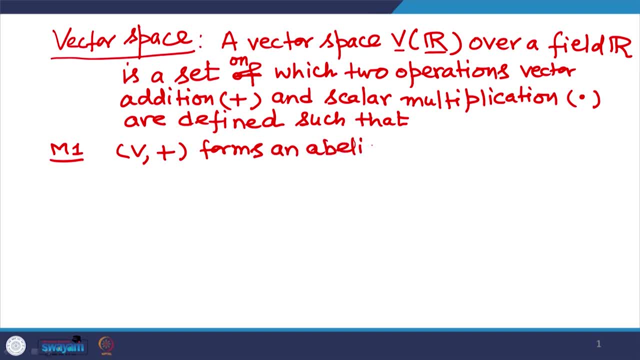 an abelian group, So here forming abelian group. Abelian group means the set of vectors. with respect to this vector, addition operation satisfy certain properties. One is closure property, another one is commutative property, associative property, existence of additive identity and existence of additive inverse. So we will make it more clear by 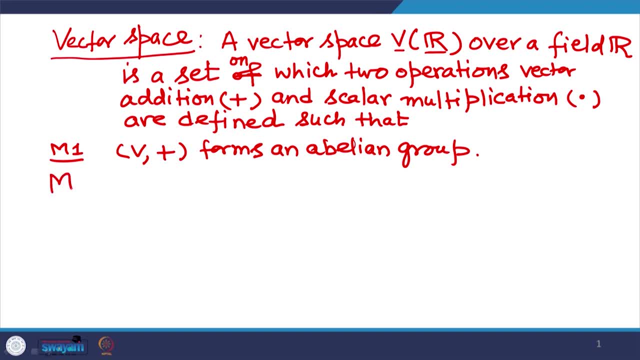 taking some example. The second property is the operation. scalar multiplication is defined between scalars, that is, the elements of the field R, and vectors, such that for all N vectors, N equal to 1, N equal to 1, 1 equal to 1 will. be equal to N, divided by 4,, 0 equal to 0,, 0, equal to 0.. So you can easily predict the prediction. So that is the first property, by definition. The second property is called the multiplication number, So that is the function, n, the function. feed product and feed product come together will be given by the given value. So next I'll go to the equation 1.. So let me take a double-and-a-half-抱ie. So let me come back to the question. 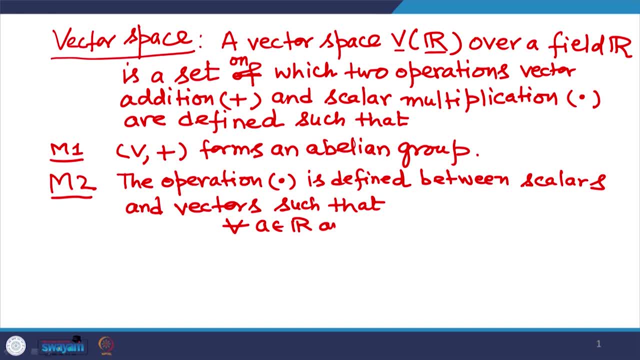 A belongs to R and V belongs to V, we have A dot. V belongs to V. The third property is for all. A belongs to R and any two vectors V. W belongs to V. we have A. multiplied with the addition of vectors V and W equals to A dot V plus A dot W. 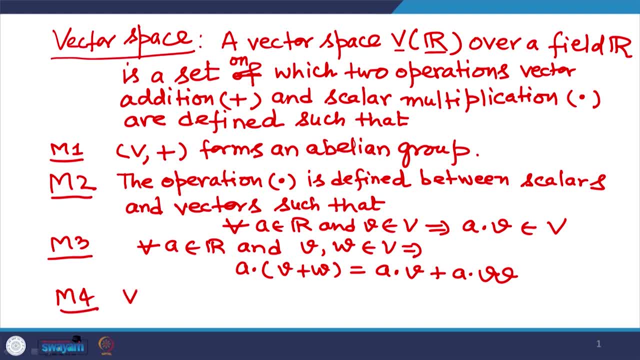 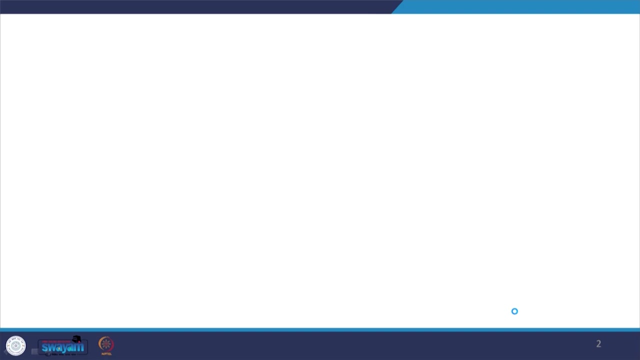 The fourth property is for any two arbitrary scalars belongs to the field R and V belongs to V. we have A plus B multiplied with V equals to A dot V plus B dot W. The fifth property is for all: A belongs to R and vector V belongs to the set V, which. 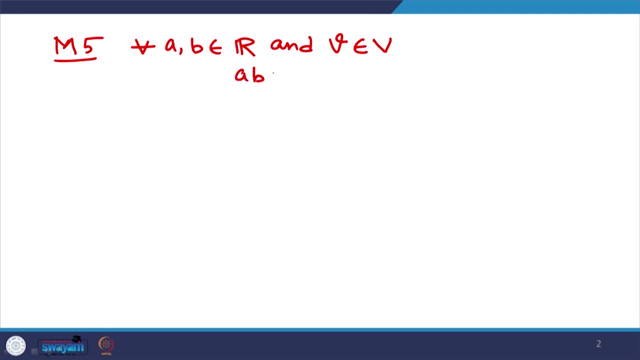 is a set of vectors. scalar multiplication with v equals to a, b dot v. So in left hand side we are multiplying a and b first and then we are multiplying this scalar to the vector v, While on right 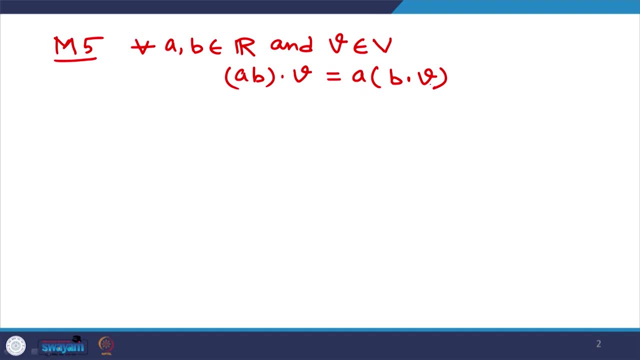 hand side, we are multiplying b first with v, and then the vector b dot v. we are multiplying with the scalar a, And the last property is that is called unitary law. So what is this unitary law? So there exists, one belongs to R, such that if you multiply this identity, 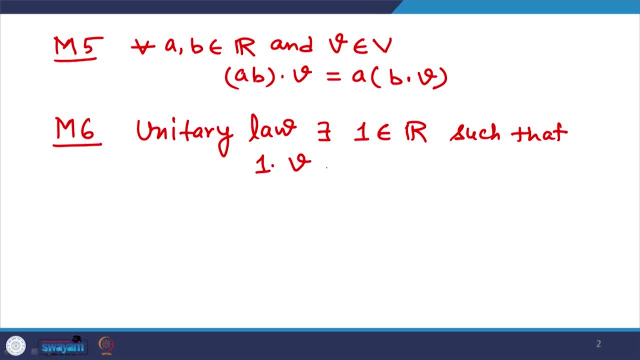 a scalar with any of the vector v belongs to V, then this is equals to V for all. v belongs to capital V. So if a set of vectors v satisfy all these six properties with respect to these two operations, then we say that V together with these two. 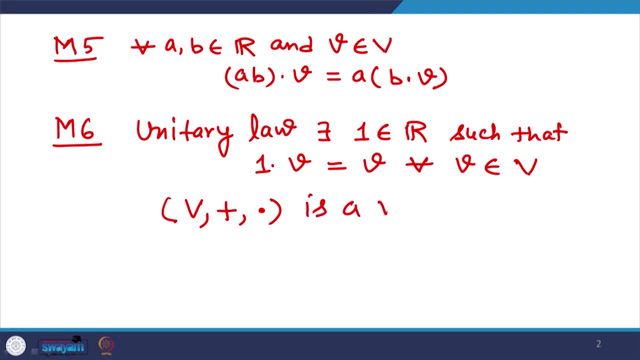 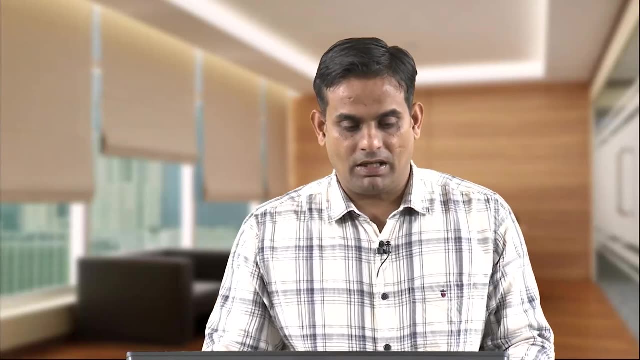 operations. So this is the unitary law. So we are multiplying a, and b is a vector space. So now we will take some of the examples of vector spaces. So my first example is coming from the vector space R 2.. 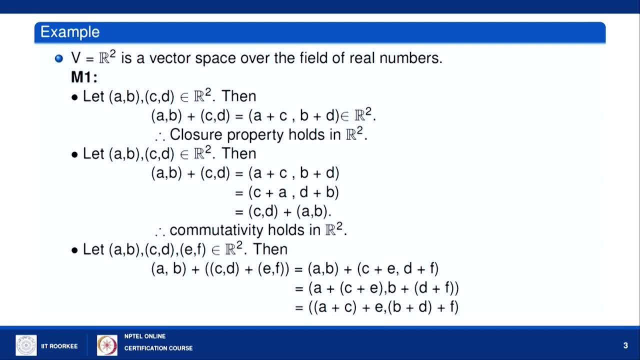 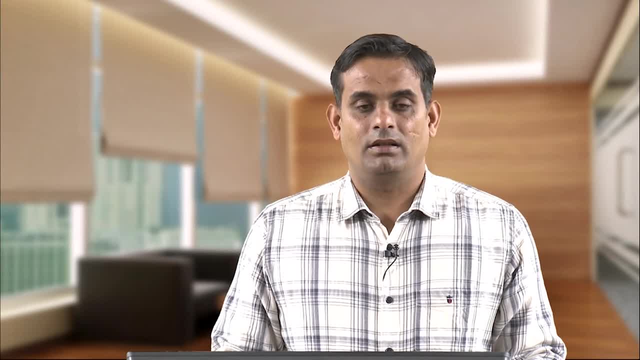 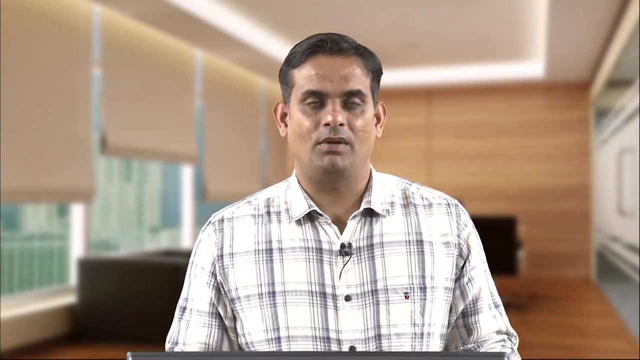 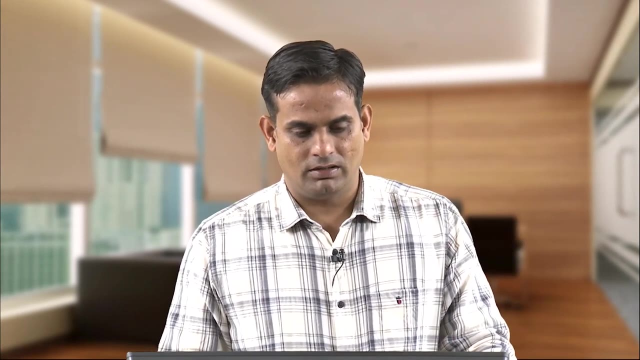 So here, R 2 is a plane- you can take it as x- y plane- and each of the point of this plane is given by a vector that is pair of point x and y, where first component is the x coordinate of that point and the second component is y coordinate of that point. So this R 2 forms: 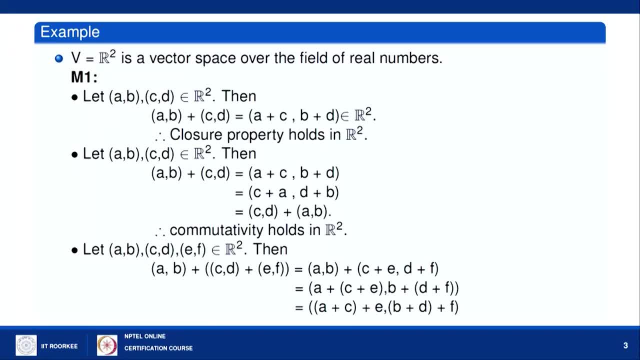 a vector space over the field of real numbers. So to check this we have to see whether it is satisfying all these six properties. So let us see property one is first. I am taking two vectors or two points in R 2 plane, that is a, b and 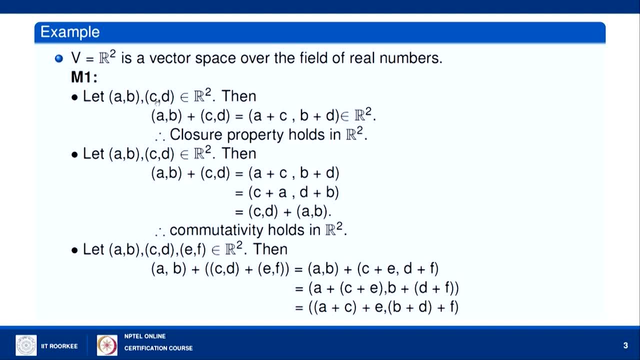 c, d. So these are two vectors, v and w. let us say, from the vector set capital V, which is R 2, then a, b plus c, d. So how we add the vector, We add the first component with the first component of the second vector and the second component of the first vector with 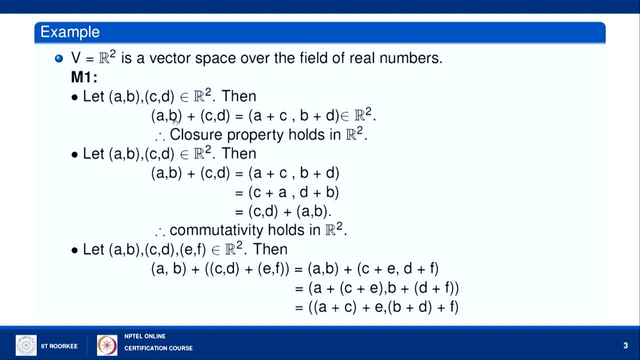 the second component of the second vector. So a, b plus c, d becomes a plus c comma, p plus d again. a plus c is a point in R 2, which is x coordinate of a point in R 2.. Similarly, p plus d is the y coordinate of a point in R 2.. 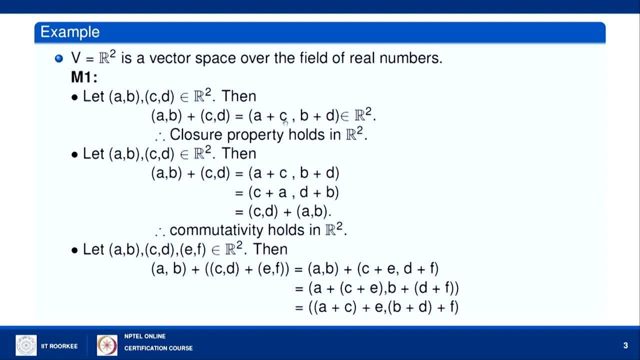 So if you add these two points again, we are getting a point in R 2.. So we can say that closure property holds in R 2.. Similarly, if I take again the a, b plus c, d, it is equals to a plus c comma, p plus d. 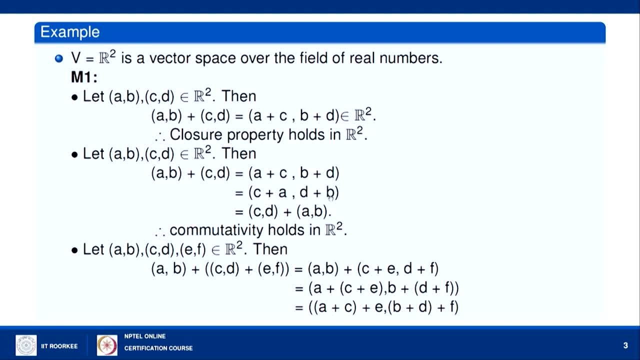 I can write a plus c as c plus a comma, d plus b, and which is nothing, just c, d plus a, b. Hence the order of the vectors in addition does not matter, and we are saying that commutative property holds in R 2. If you take three vectors, let us say a, b, c, d and e, f, Then first I: 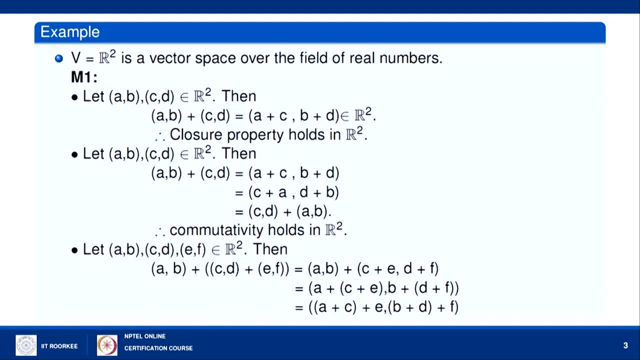 am adding here c d plus e, f, and then, whatever result I am getting, I am adding a b into it, So it will become a b. In fact it will become c? b. So I have written that c- b is equal to c d plus b into c comma. 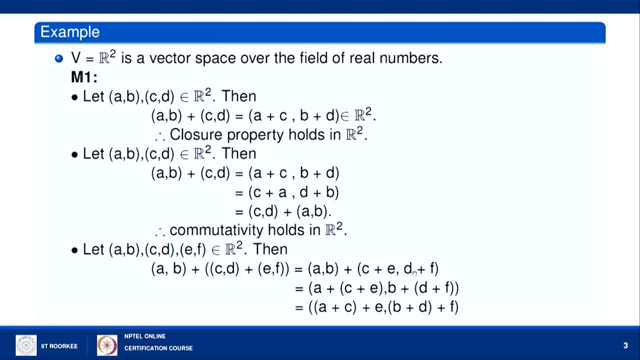 c plus c plus e, comma d plus f. Now I can write it a plus c plus e, comma b plus d plus f. Since these are scalars, these are real numbers, so they satisfy the associative property. so a plus c plus e, I can write a plus c plus e. Similarly, b plus d plus f, I can write: 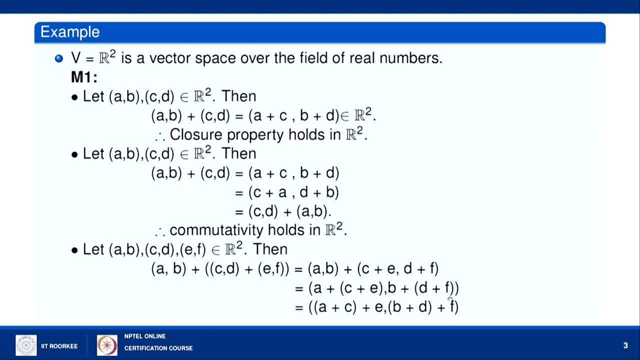 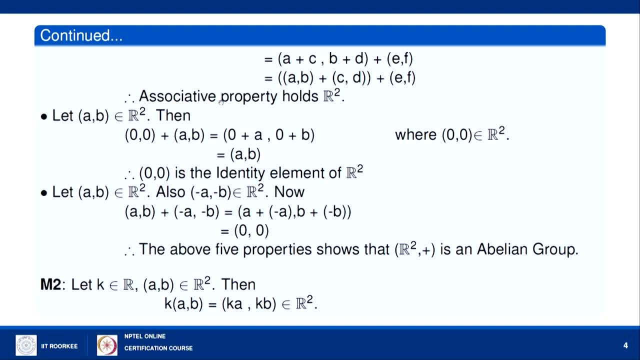 b plus d plus f, So hence it becomes f e plus c, d plus e, f. Hence associative property holds in R2.. Further, if you take the origin of R2 plane, that is 0, 0.. So if you add this, 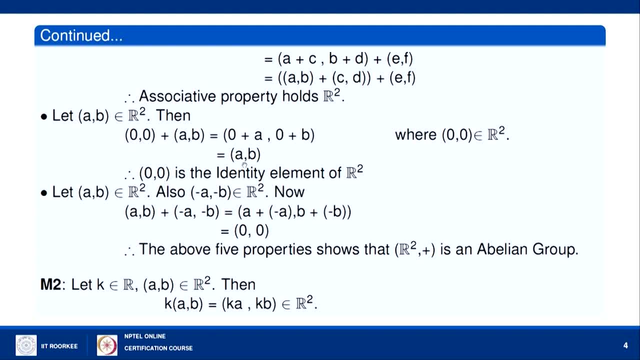 in any vector a, b, the result will come out to be a, b only. So hence 0, 0 is an element of R2.. And it is identity element. So existence of identity holds here. Next, if you take a, b, then certainly there will be minus a, minus b. Also will be there R2. and if we add these, 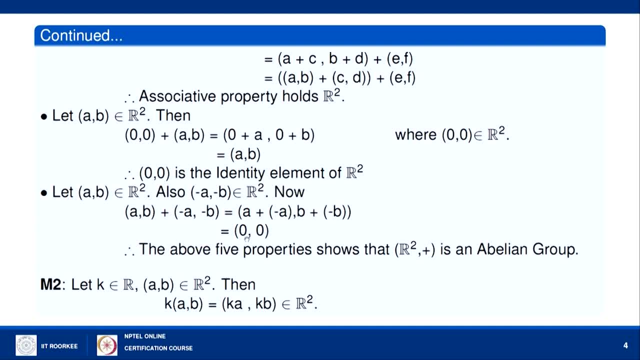 two points, then result will come out to be 0: 0, which is nothing, just additive identity of R2.. Hence the existence of additive inverse is 0: 0.. So it is 0: 0.. inverse whole in R 2.. So these points satisfy and they implies that R 2 plus forms an abelian. 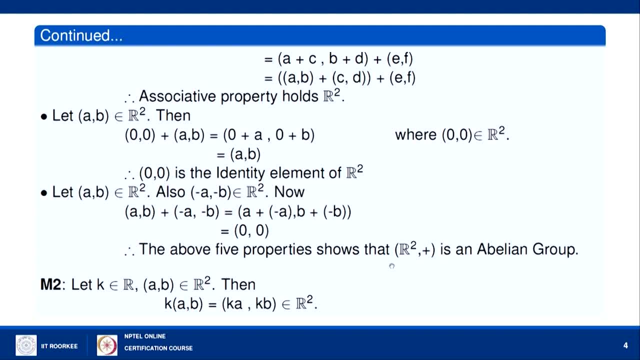 group. So this is the first property which we have defined in the definition of vector space. Now come to rest of the properties. So my second property was there that if you are having a scalar and a vector, then the scalar multiplication between them also an element. 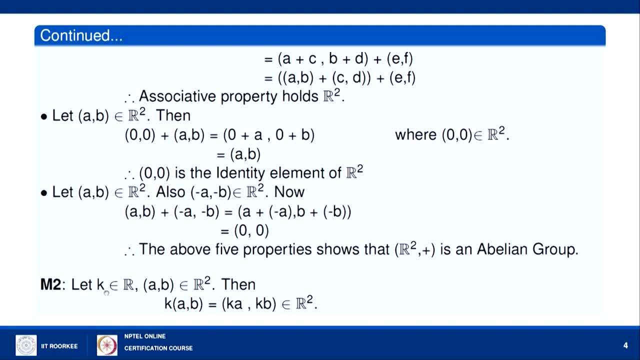 of the set R 2.. So I am taking here: k belongs to R, which is a scalar. a, b is a vector from R 2, then k multiply with a, b will become k a comma, k b. So again: k a, comma, k b is a vector from R 2.. 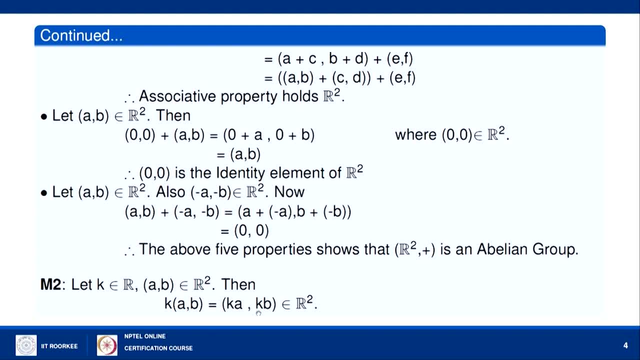 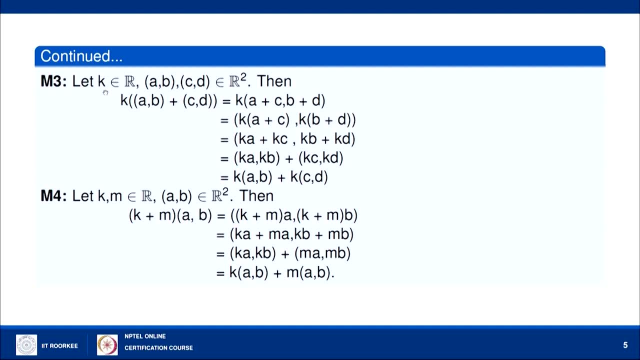 So k is an element in R 2 and hence the second property holds. So now come to third property. I am taking a scalar k here and two vectors given by a, b and c d. Then the multiplication of k with the addition of these two vectors, a b and c d, can be written in this form: k. 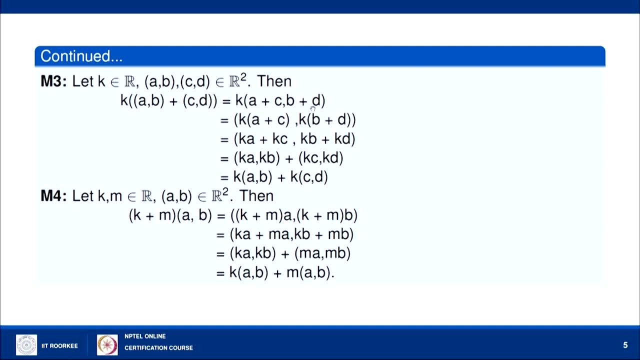 times a plus c comma b, So k a plus c comma, k b plus d. I can take k inside, So k a plus c comma, k b plus d, which is k a plus k c comma, k b plus k d. This I can write k a comma k b plus k c comma. 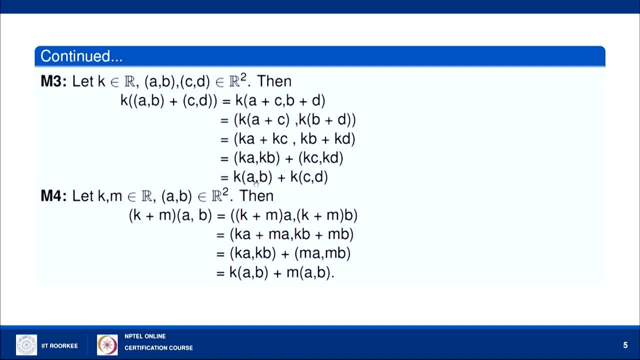 k d, and which is nothing but k times a b plus k times c d. So hence third property hold in R 2.. With respect to the operations, So I am taking k a plus c comma, k b plus c d, So k a plus c comma, k b plus c d So. 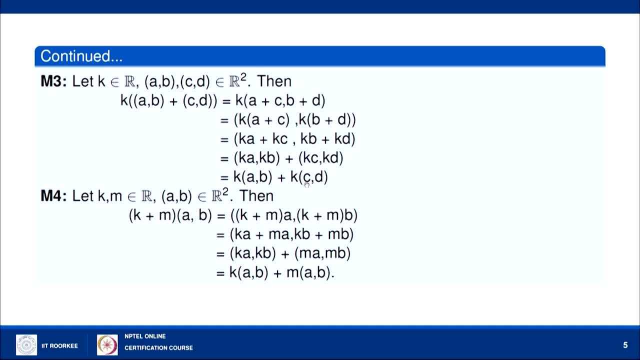 this is a vector addition and scalar multiplication. Now come to the fourth property. I am taking two scalars, k and m. Now come to fourth property. I am taking two scalars, k and m, from the field R and a vector a, b from the set of vectors. 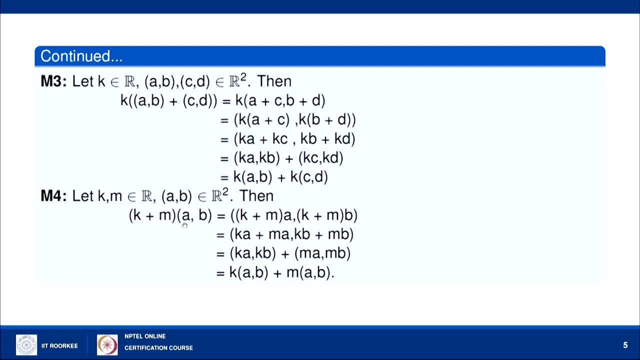 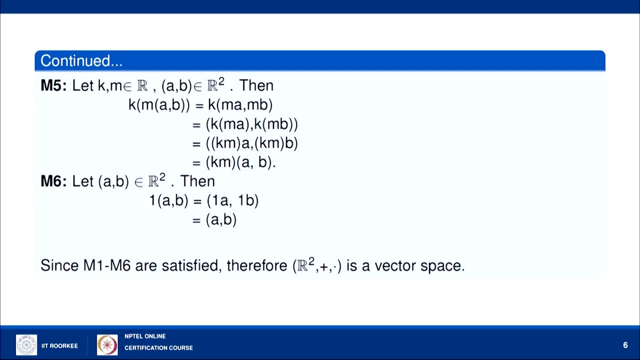 R 2. Then k plus m times a b can be seen as k times a, b plus m times c comma, c comma M times AB. So hence fourth property holds in R 2.. Now come to fifth property. So here: 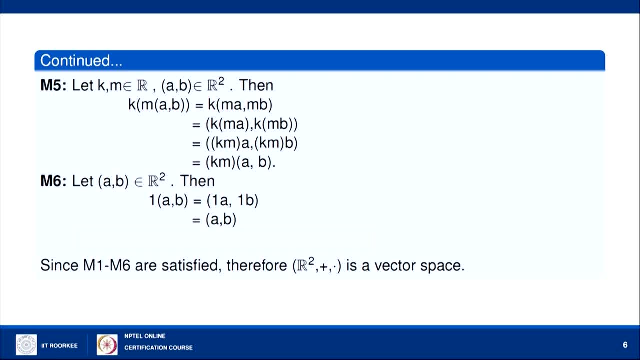 again. I am taking two scalars from the field of real numbers, K and M, and a vector element AB from R 2. Then K times M times A comma B can be written as K M A, comma M B, which is nothing, just I can take K inside again the bracket K times M A comma K times M B. 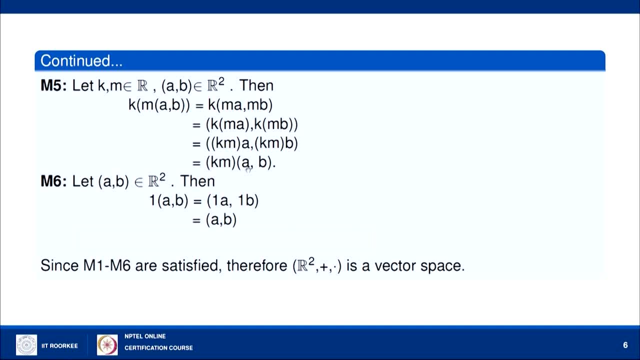 and this finally comes out to be K M times A, comma B, which is the fifth property. Further, you know that 1. Belongs to the field R means 1 is a real number and if you multiply 1 with any vector, AB it. 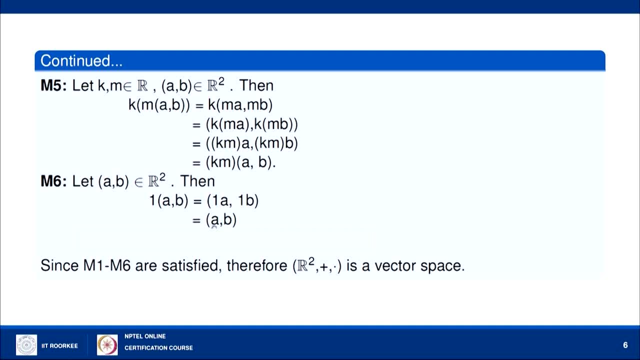 will be 1 comma A comma, 1 comma B, and it is nothing. just if you multiply 1 to any real number, the real number will remain same. So it is equals to A comma B. here unitary property holds. So here all M 1 to M 6 are satisfied, and 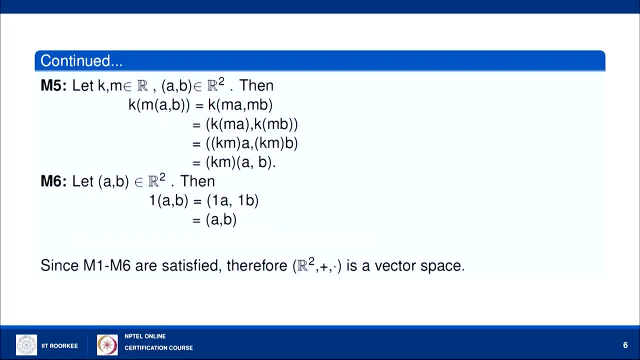 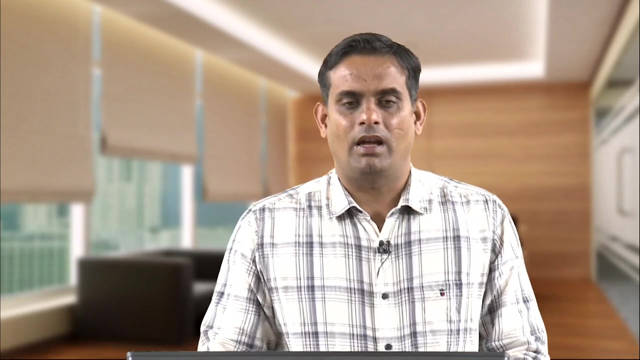 then, Therefore, we can say: R 2 on the field of real number, with respect to the operation set, addition of vectors and scalar multiplication is a vector space. So this is an example of R 2.. Similarly, we can show that R 3 is also a vector space and any set of vectors. 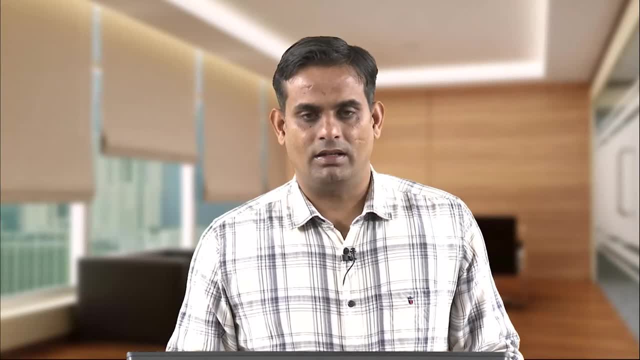 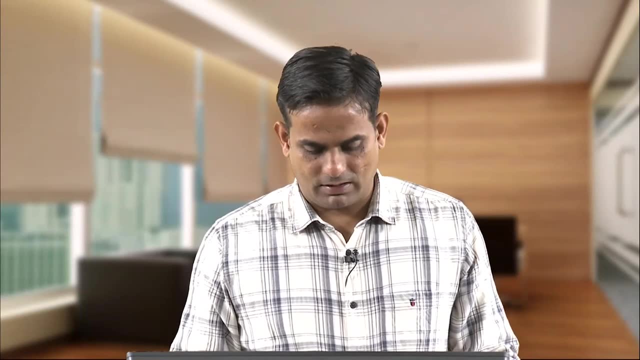 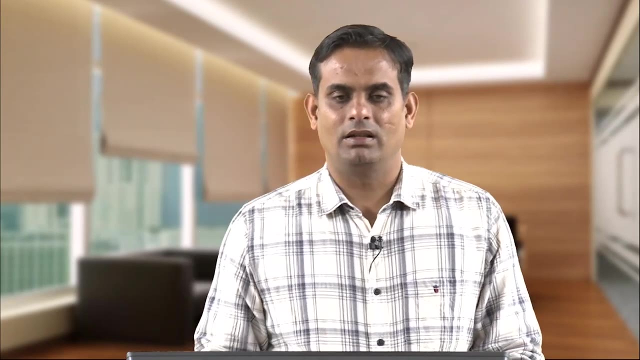 like R n. So each vector is having the n components: x 1, x 2, up to x n also forms a vector space. So this we have talked about, R 2, R 3 and R n, these kind of vector spaces, those are. 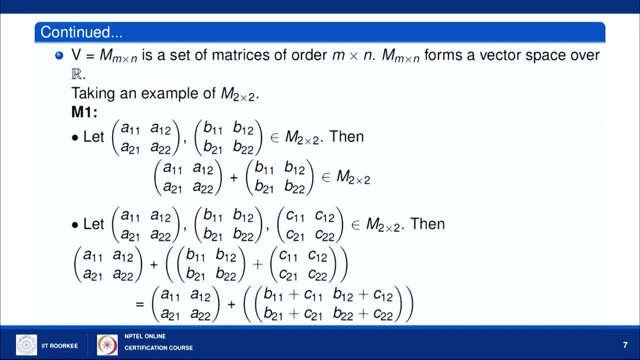 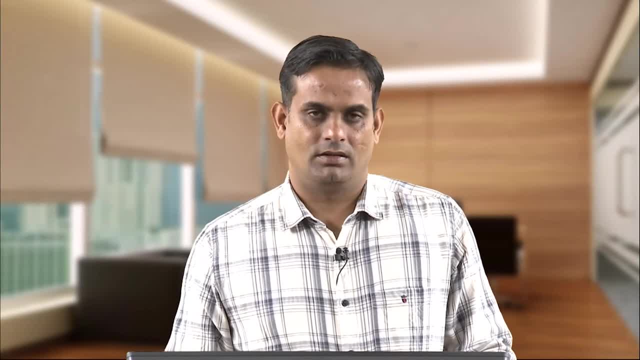 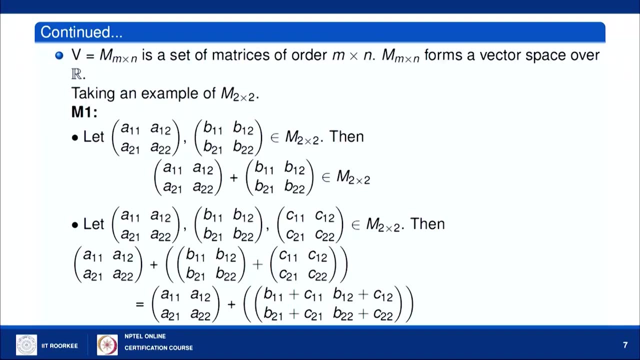 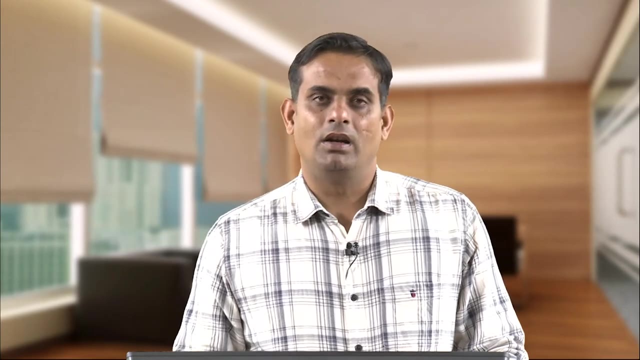 very common in machine learning. but the same time the set of matrices of order m by n. So where m and n are real integers, So integers in fact. So any matrix of order m by n forms a vector space over the usual. 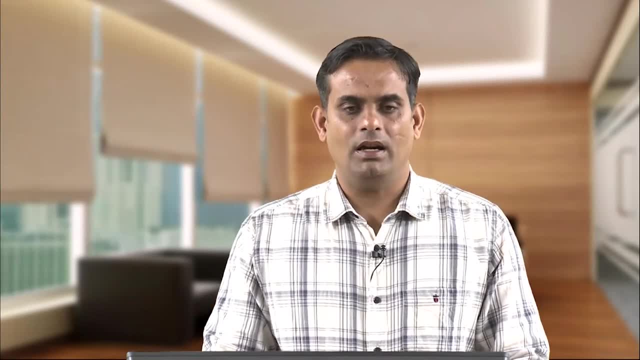 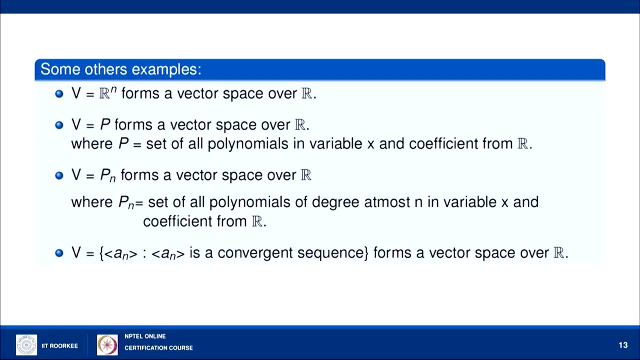 addition of matrices and the scalar multiplication. So there are many other examples of vector spaces. as I told you, R? n forms a vector space over the field R. If you take the set of vectors of all polynomials in variable x and having real coefficient, then this set also forms: 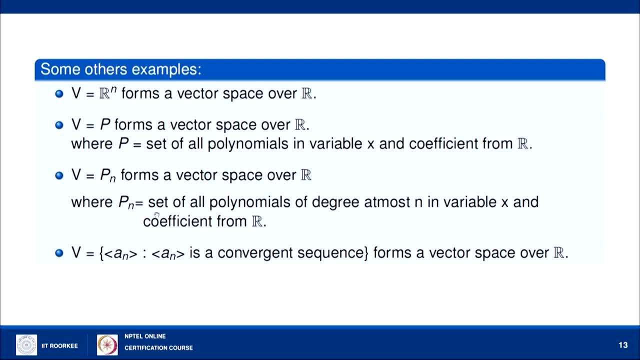 a vector space over the field R. Similarly, if you take a set of all polynomials of degree, at most n, So degree either n or less than n in variable x and having real coefficient, then this set also forms a vector space over the field of real numbers. 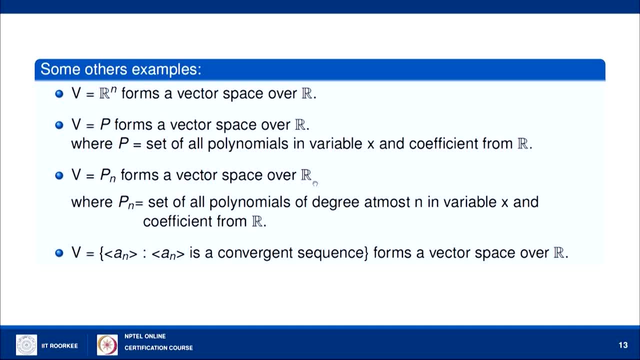 With respect to the operations usual polynomial addition and scalar multiplication. If you take V as the set of all convergent sequences, then this set also forms a vector space over the field of real numbers where the operations are usual, sequence addition and scalar multiplication. So so far we have seen many examples of vector spaces. Let us 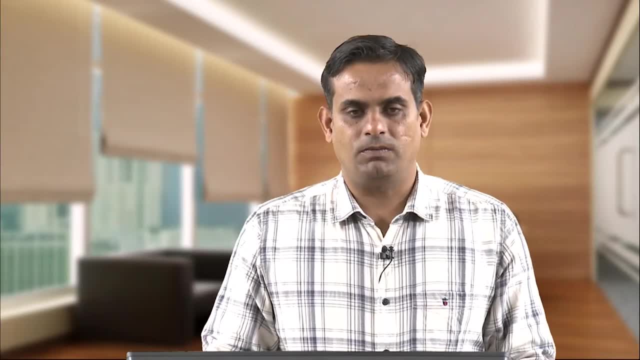 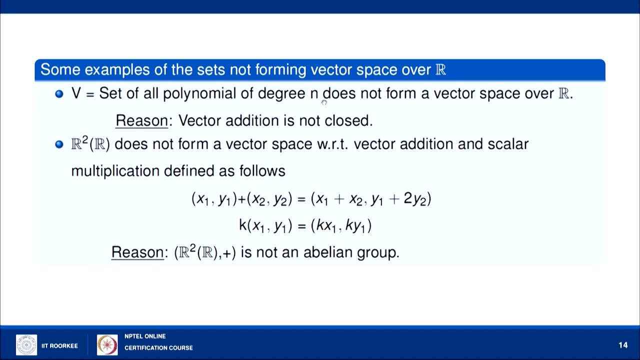 see some of the set. those do not form vector spaces. So my first example is: set of all polynomials of degree n does not form a vector space over R. Why? Because vector addition is not closed. So if you want to see this, So let us say two elements from V. So here: 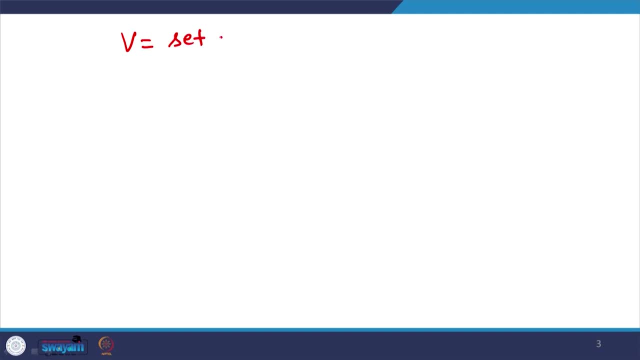 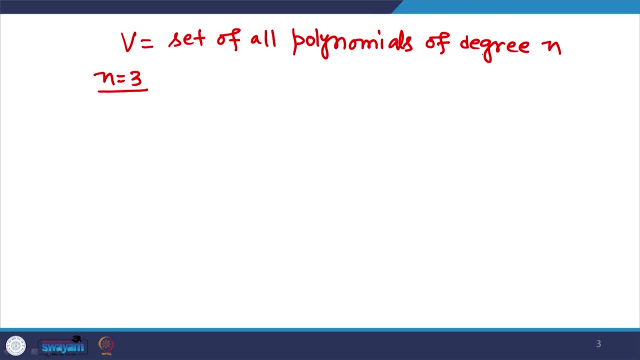 V as the set of all polynomials of degree 3.. So let us take two vector, two elements from this set, or two vectors from this set. So let us say V 1.. So V 1 I am taking. let us say 2 x cube plus 5 x square plus x plus. 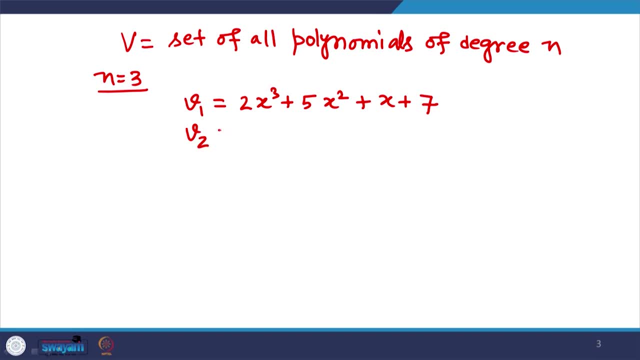 7, and I am taking another vector: minus 2 x cube, plus 3 x square, plus 4 x plus 1. So V is the two polynomials of degree 3. So it is an element of V. It is an element of V. 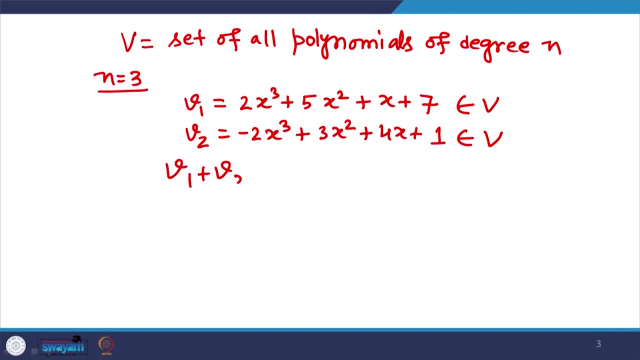 Now if I take V 1 plus V 2.. So what will be V 1 plus V 2?? So it will become 8 x square, because x cube term will be cancelled, plus 5, x plus 8 and it is a polynomial of degree. 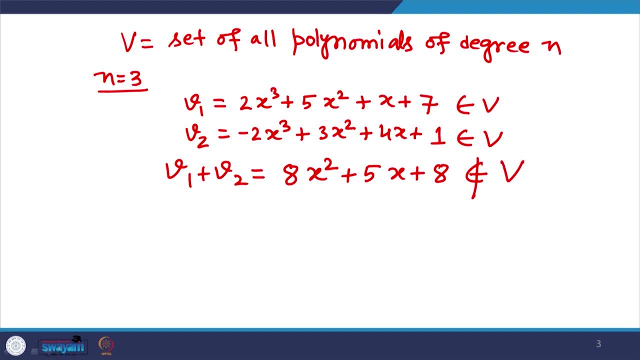 2. So what will be? our vector is 12 over 2, five x plus 2, and again helping us out. So hence it is not an element of V, So hence this set do not form a vector space, So closure. 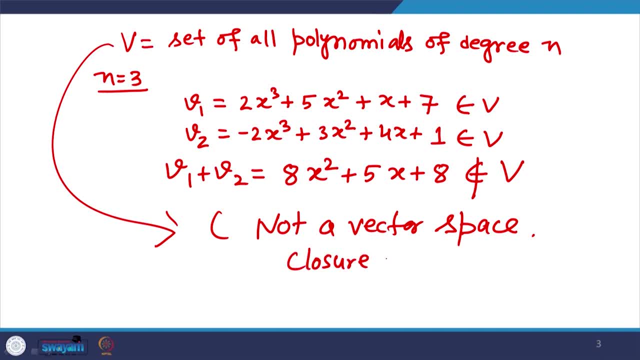 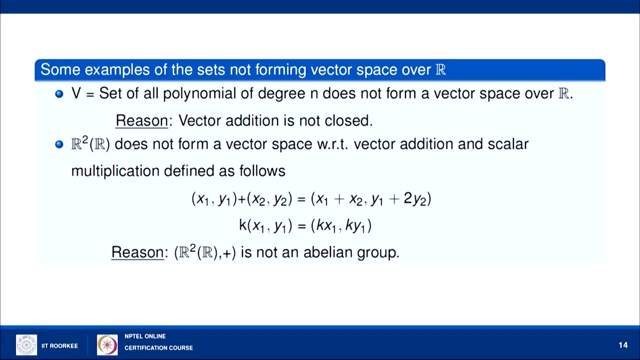 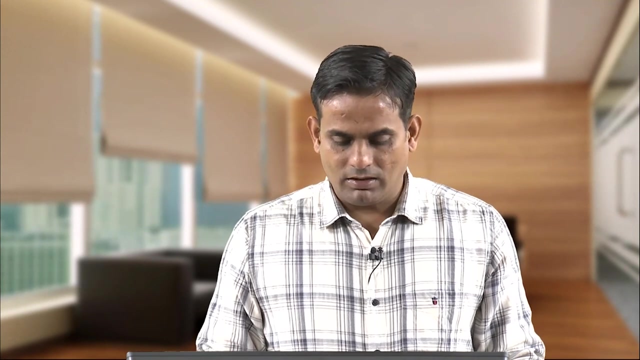 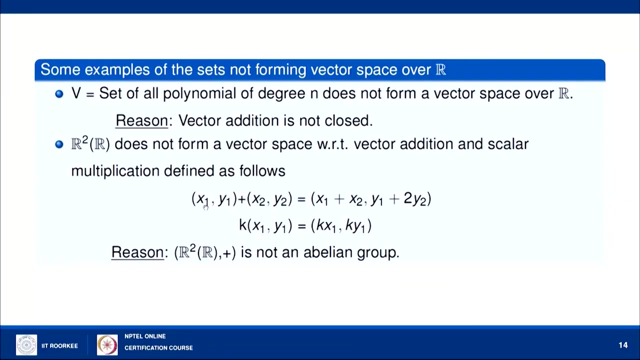 property. Similarly, if you take R to R, we have seen in earlier example that if you take the usual addition of vectors in R 2 and the usual multiplication of real numbers, then it forms a vector space. But if you define your vector addition and scalar multiplication in this way, like if 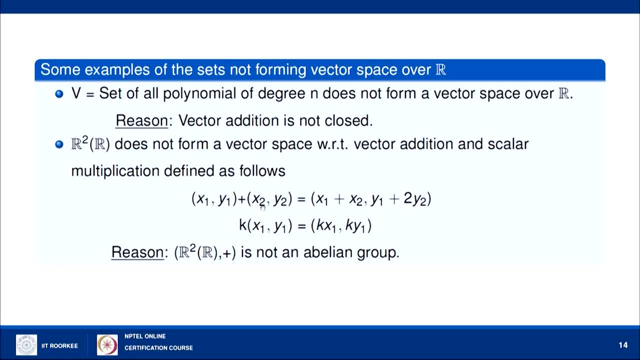 you are having vector x 1 y 1 from R 2 and another vector x 2 y 2 from R 2, then their sum is x 1 plus x 2, comma: y 1 plus 2 y 2.. In usual case it will be y 1 plus y 2, but 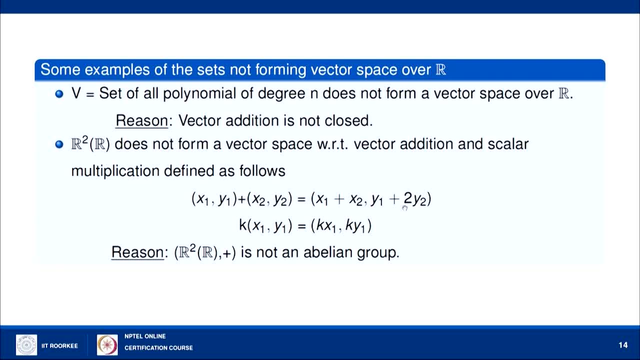 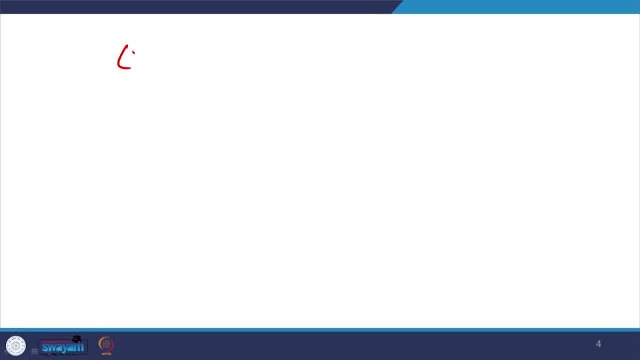 we are defining this operation in this way. R 1 can define. But if you are defining in this way, then what we will see? that So x 1 comma y 1 plus x 2 comma y 2.. So these are 2 vectors from R 2 and we are defining. 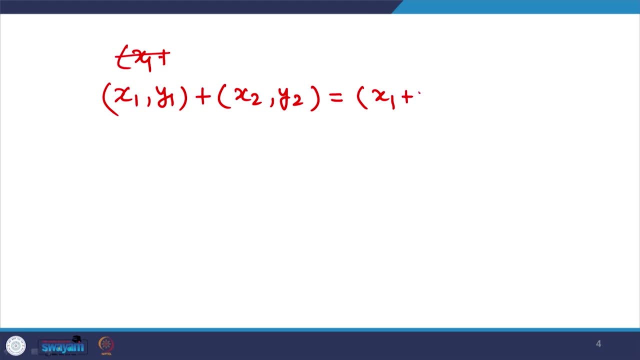 their vector addition as x 1 plus x 2.. y 1 plus 2 y 2.. Now if I take the reverse order x 2 y 2 plus x 1 y 1, then it will become x 1 plus x 2. first component will be the same as in the previous case. However, in the second 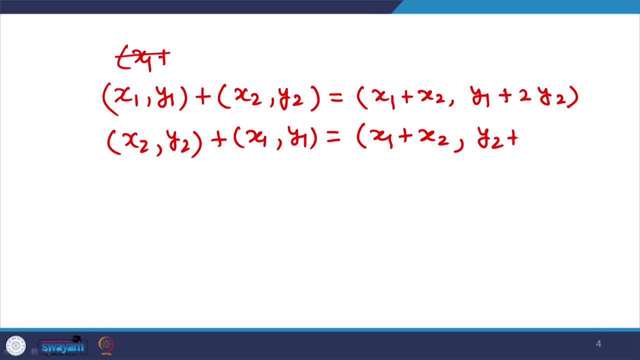 case it will become y 2 plus 2 y 1.. So now this second y coordinate of these vectors. so it is y 1 plus 2 y 2, it is y 2 plus 2 y 2 y 1, sorry, y 2 plus 2 y 1, hence both are. 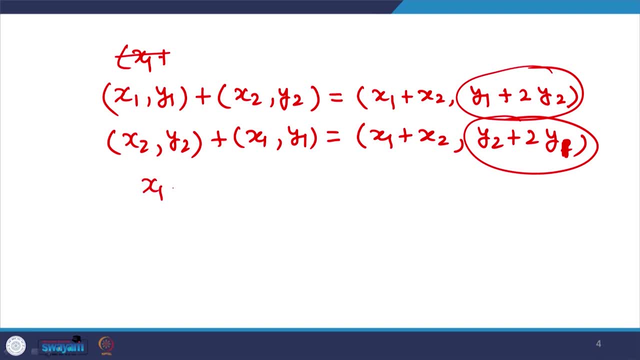 not equal. So what we can say: x 1 y 1 plus x 2 y 2 plus x 1 y 1 not equals to x 2 y 2 plus x 1 y 1, in general for all vectors in R 2.. So what? 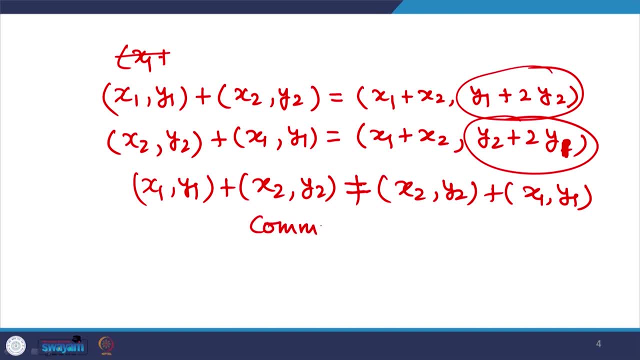 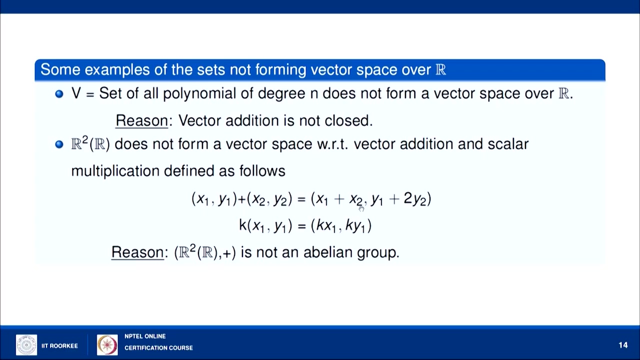 I can say that commutative property Does not hold So. hence, if you are defining your vector addition in this way, by this operation, then it R. 2 on the field of real numbers does. 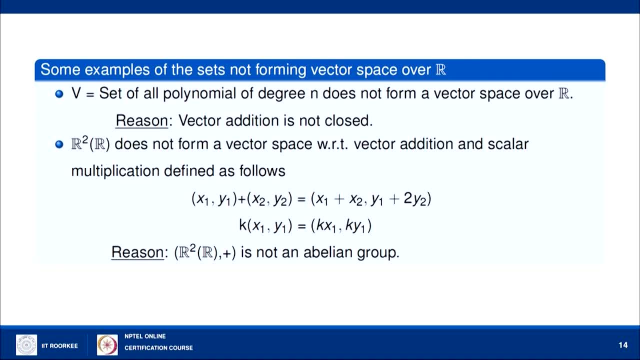 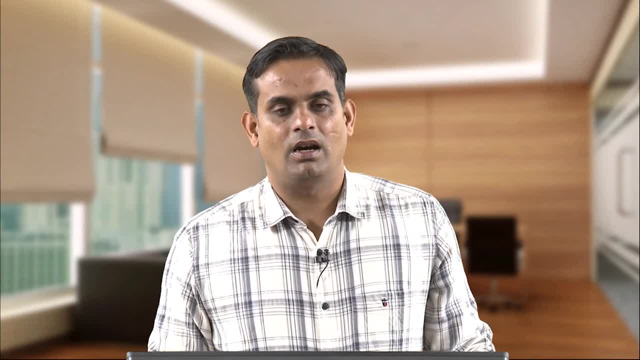 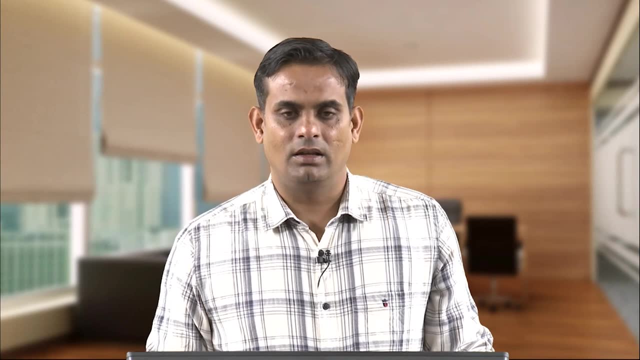 not form a vector space. So what we can say from here, the only set is not important in the definition of vector space, but the operations also, how you are defining your operations, operations For a particular set. one set of operations will satisfy all the six properties. 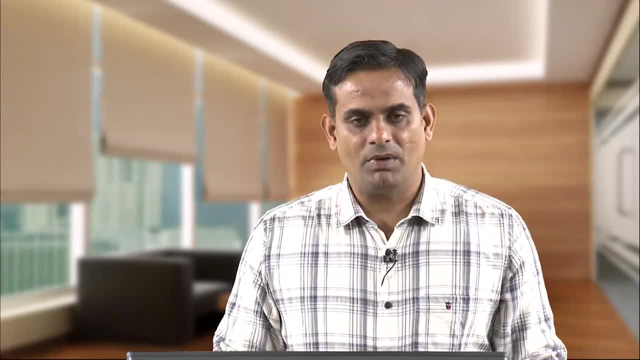 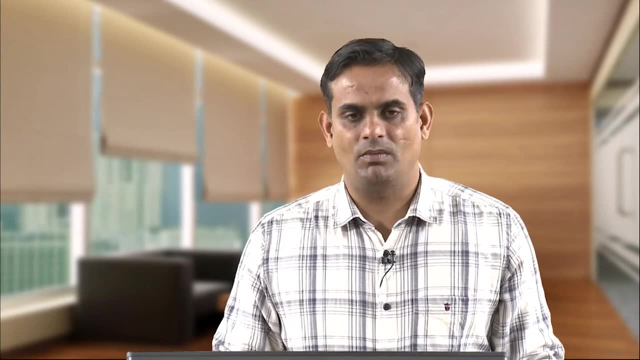 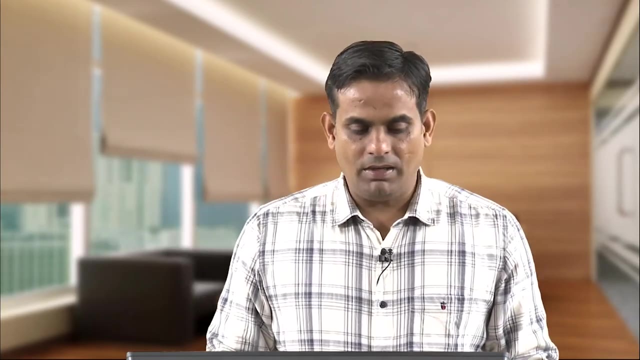 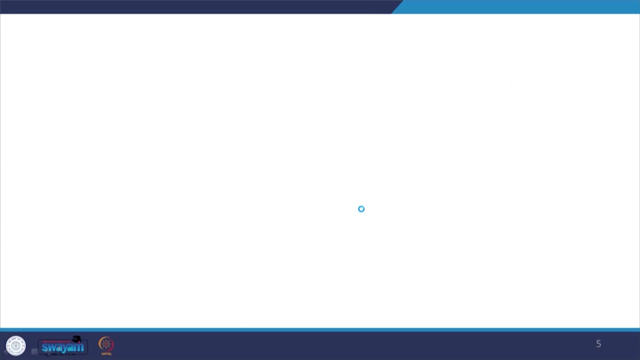 of vector space. but if you change the operation, it may happen that the particular set does not form a vector space, So you have to be careful in this case. Now we are coming to geometric interpretation of R 2 and R 3.. 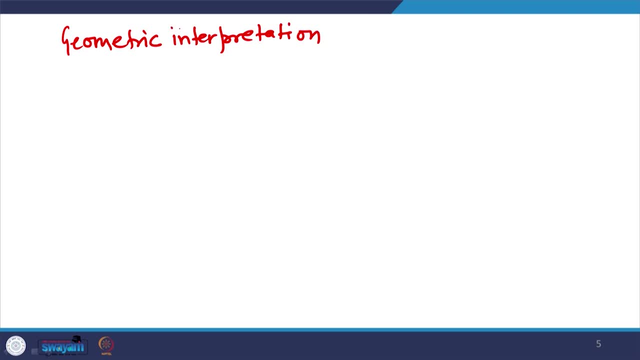 So R 2 and R 3 are geometric interpretations. Now we are coming to geometric interpretation of R 2 and R 3.. So what we can have for n equals to 1,, 2 or 3, the space R n has a very useful dimension. 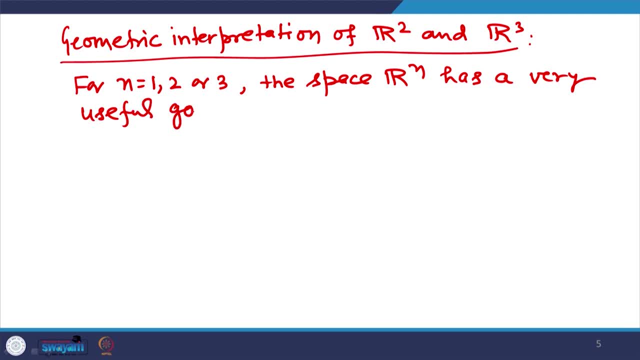 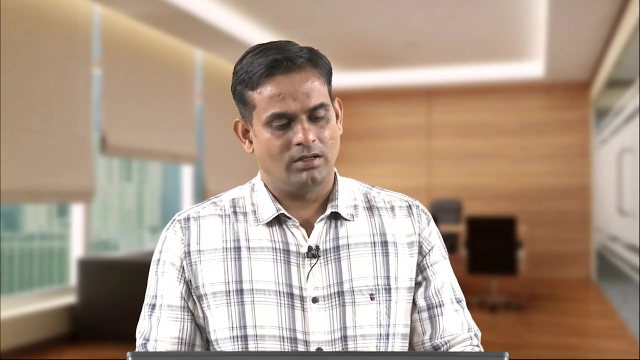 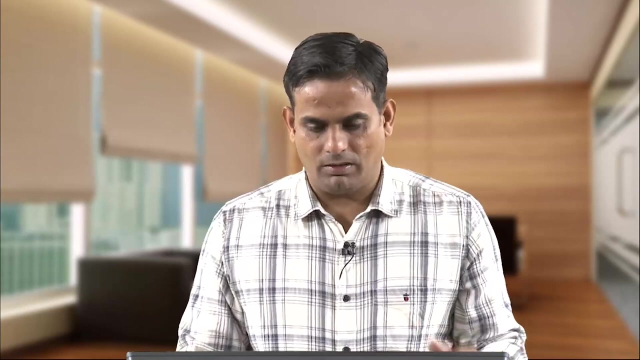 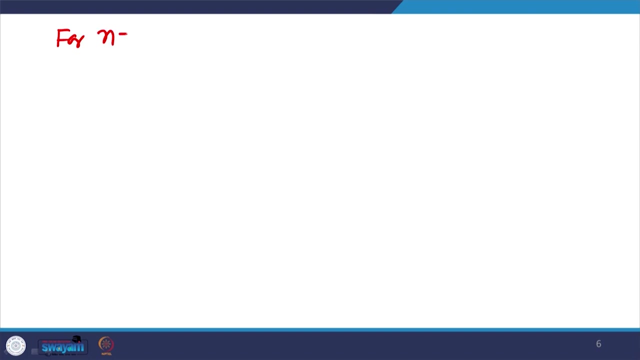 tool geometric interpretation For n greater than 3. we cannot see in general, but for n equals to 1,, 2 or 3, we can have this beautiful geometric interpretation How. Let me explain it. So for n equals to 1, we are having the set V equals to R and the vectors will be like: 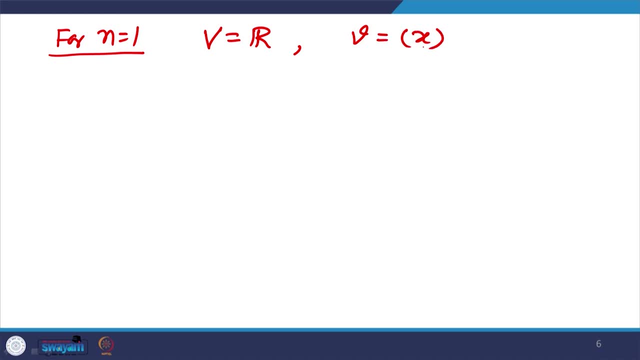 V equals to x. So how you will see geometrically this vector. So on the real line you will be having the origin. let us say 0 here, and then 1, 2, 3 and so on. similarly, here, minus 1, minus. 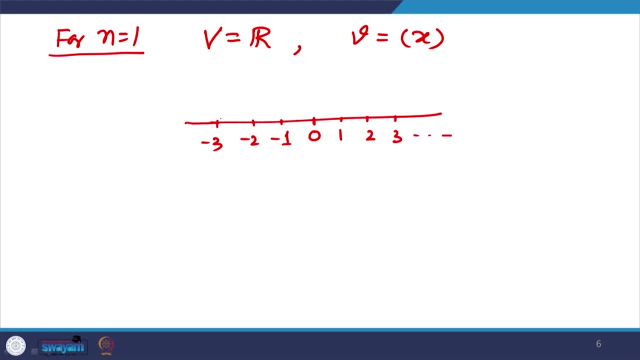 2 minus 3 and so on. So we are having this real line. Now, if we are having a vector, let us say V equals to x equals to 5.. So what will be this? x, x equals to 5.. So let us say 5 is here, So the tail of this vector will be here at 0. 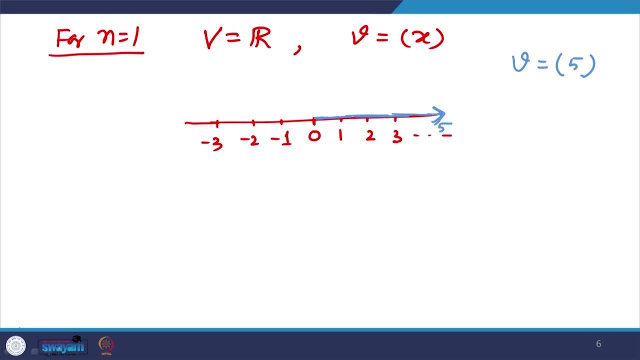 and then we are having the head here at 5.. So this is the vector: v equals to 5.. Similarly, if I am having something like v equals to minus 2.. So v equals to minus 2 will be again, tail will be here and I will be having this. So, by the green color, I am showing you the 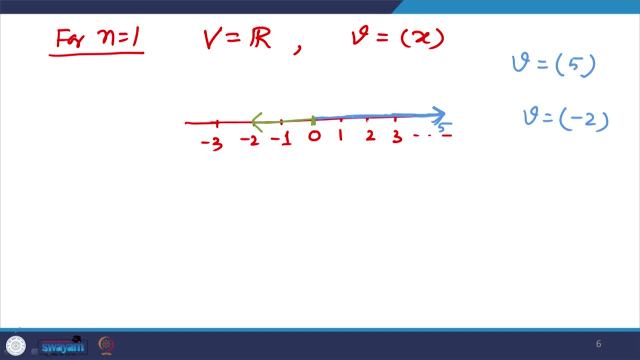 vector v equals to minus 2 and by the blue color I am showing you, the vector v equals to 5.. Similarly, for n equals to 2.. So now it is set of: vector is r, 2 and the vector will be something like v equals to 2.. 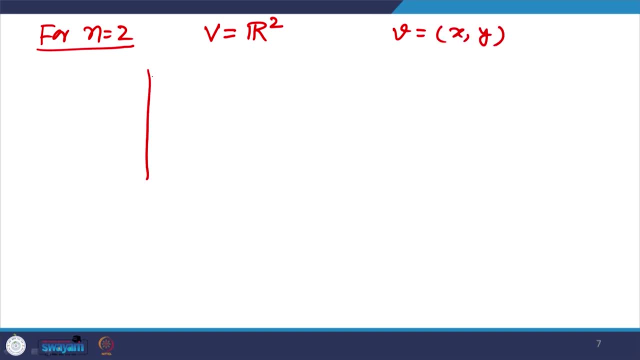 So in coordinate plane x- y this vector will be having tail at the origin and suppose this is the point x- y. So this is straight line joining the origin and the point x- y will show the vector v. So n equals to 3. we are having the three-dimensional coordinate plane, So let us say x, y and z. 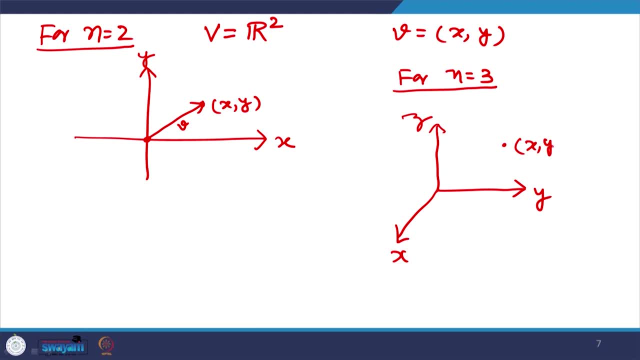 and I am having a point. let us say x y, z here. So again, it will be a line in 3D having tail at the origin. So this is my vector. v equals to x y z. So if you are having two vectors, let us say v. 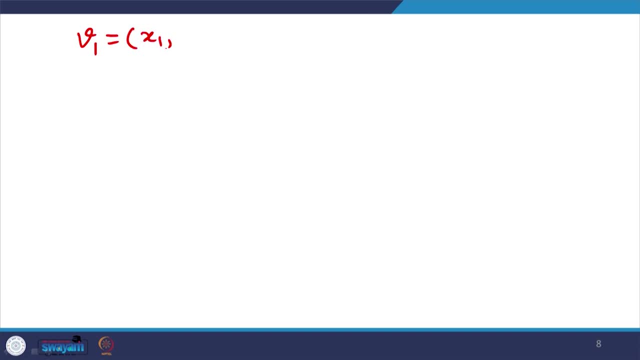 1 equals to x 1, y 1, z 1 and v 2 equals to 1.. So this is my vector. v equals to 1.. So 2, y 2, z 2- both are in R 3, then v 1 plus v 2 will be x 1 plus x 2, y 1 plus y 2, and 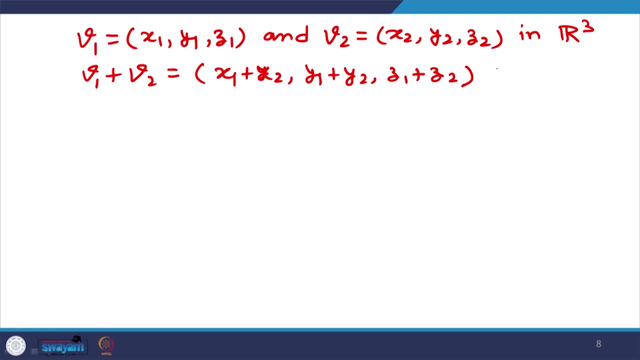 z 1 plus z 2, which is again a vector in R 3, because R 3 forms a vector space. and how to see these. So let us say: this is my vector v 1,, this is my vector v 2, then the sum of 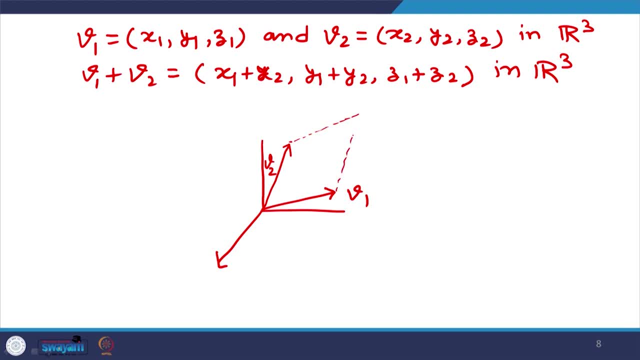 v 1 plus v 2 is given by The diagonal of this parallelogram. So this is my v 1 plus v 2.. One more important remark here: if v 1, v 2 and v 3 are linearly independent, v 1 and v 2 are linearly independent. So 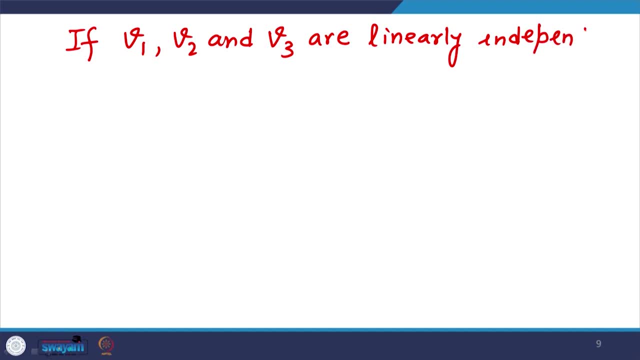 what is the meaning of geometrically of this sentence? So it means v 1 and v 2 are not collinear And the vector v 3 is a vector of the same type. I mean that is the vector of the same type. So v 1, v 2 and v 2 are not collinear. The vector of the same type is V 1, or vector of the same type is V 3.. We can also divide it same right. So this is the definition of V 1 and V 2.. So, and what is the meaning? 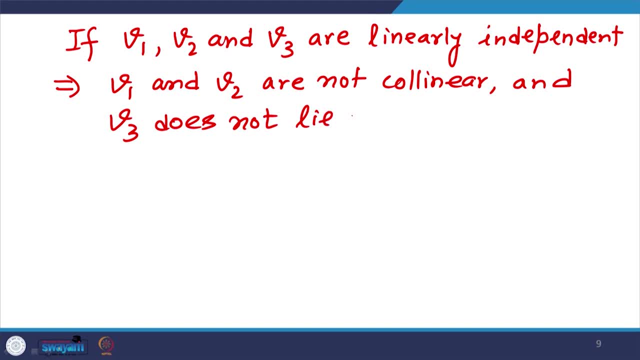 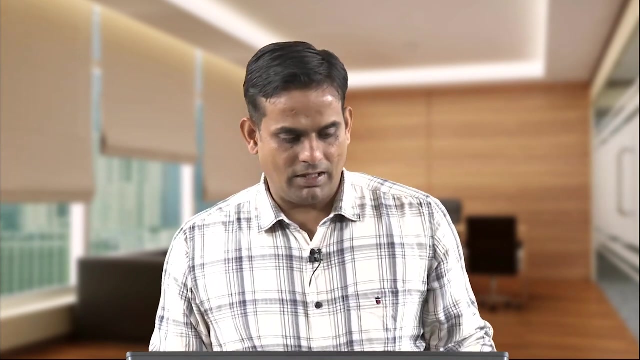 of this sentence. So it means V 1 and V 2 are not collinear. So we have a vector of, the does not lie in the plane of V 1 and V 2.. So these are some geometric interpretation of vectors in R 2, R 3.. Similarly we are having Euclidean space, R n, where we are having 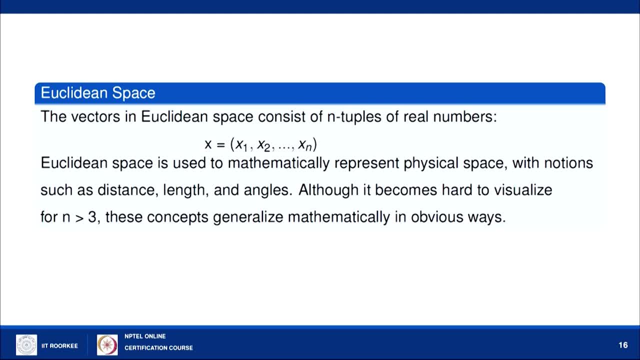 the vectors coming from n tuples. like a vector, x is x 1, x 2 up to x n. So Euclidean space is used to mathematically represent physical space with notions such as distance length angles, although it becomes hard to visualize for any when n is greater than 3. That is.